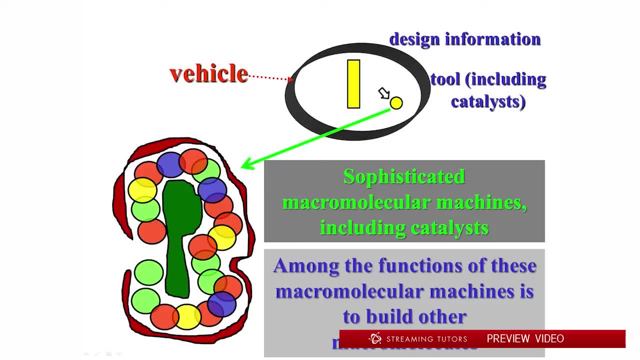 carbohydrates are one of several classes of those other macromolecules- lipids being the other major one which we'll talk about elsewhere- and our goal today is just to understand the basics of carbohydrates, how they're made, what the nomenclature for describing them is. some of their elementary 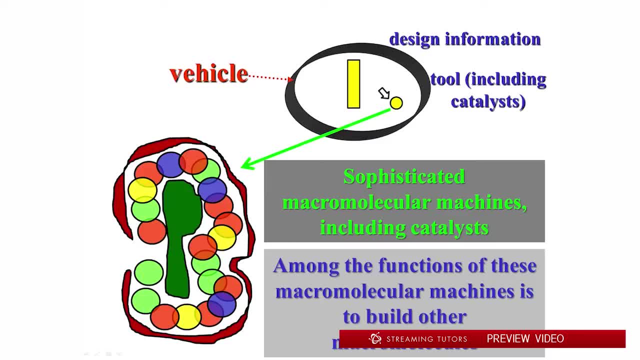 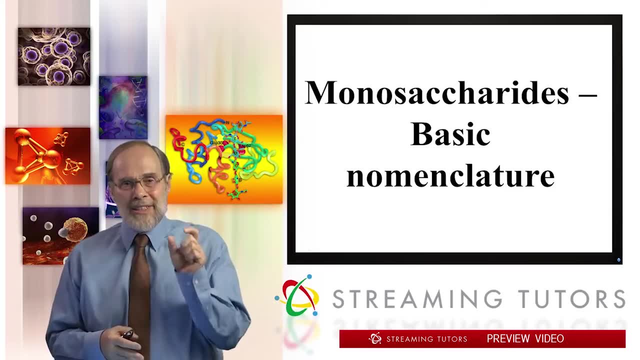 factors and then look at a couple of their biological actions, that is, when they show up in organisms and what the implications of their presence are. so let's start with the basics: monosaccharides, single monomer units, so the mono should key that to you here. these: 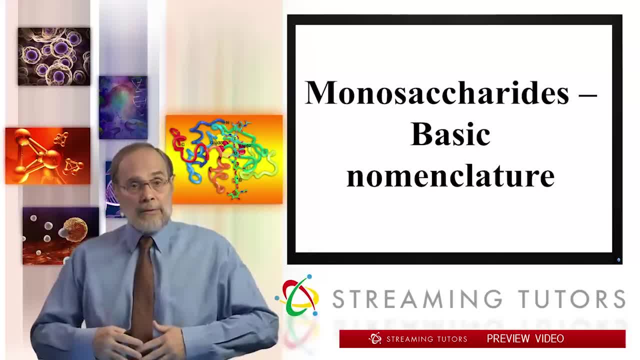 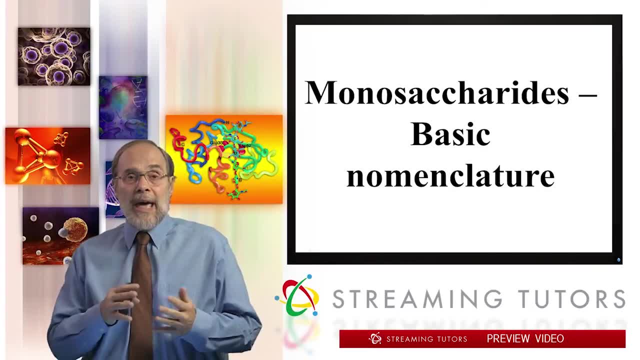 are polymers like proteins or polymers like nucleic acids are polymers, but these polymers are not genetically encoded directly. they're built by genetically encoded tools, catalysts that build them from scratch. So they're especially well-named. So they're especially well-named. 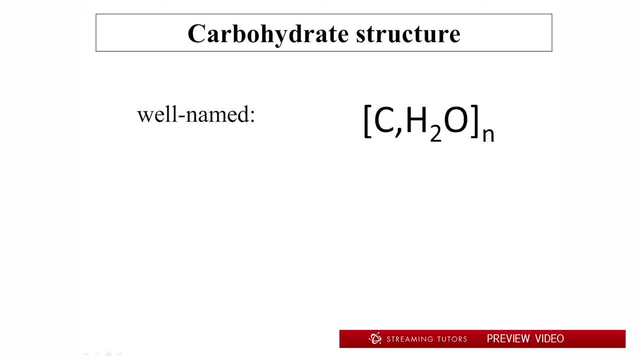 So most of the basic carbohydrates- ones that we'll talk about shortly in segments to follow on metabolism, like glucose, for example- are very well named by the name carbohydrate, That is. their empirical chemical formula is one water per carbon, That is one H2O, one carbon atom times N. 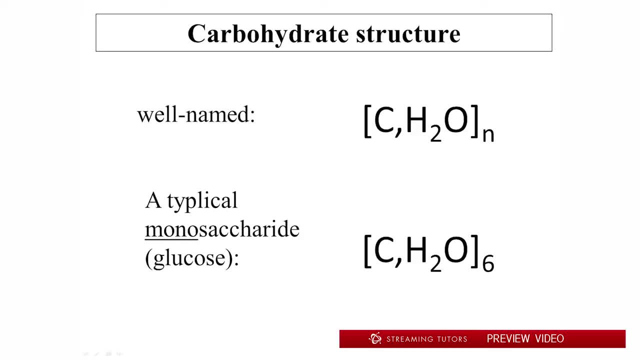 And a particularly typical monosaccharide, glucose. as you'll see, it's all over the place in metabolism and biological structure. It's probably the most common monomer, biological monomer- in the biosphere, for reasons that will emerge. 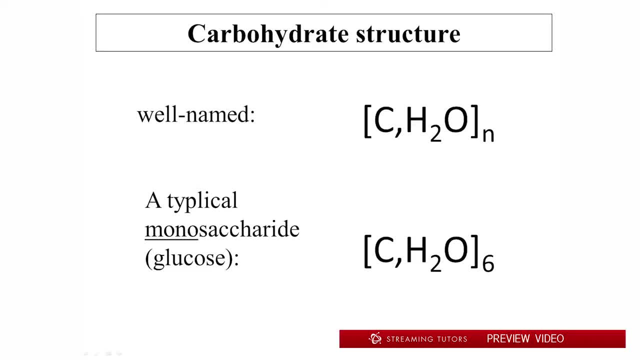 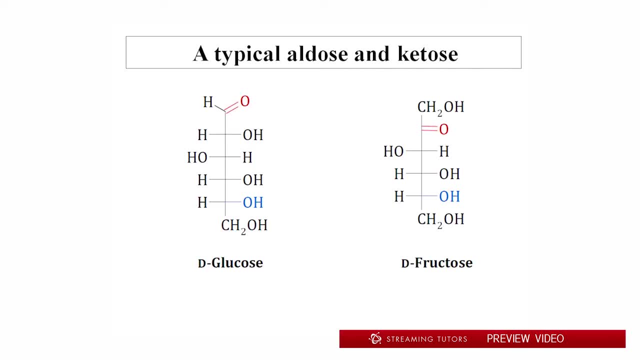 And it in fact has CH2O times 6 as its empirical formula. It's a stoichiometric, chemical stoichiometry. So let's begin by the first crucial element of nomenclature, That is, monosaccharides. single sugar units are either ketoses or aldoses. 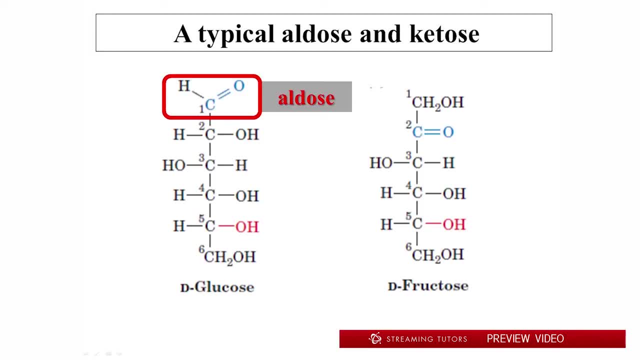 Let's illustrate what that is. So glucose is in fact an aldose. What does that mean? It means that the carbonyl group characteristic of monosaccharides- so all conventional monosaccharides have a carbonyl group- one of their properties. 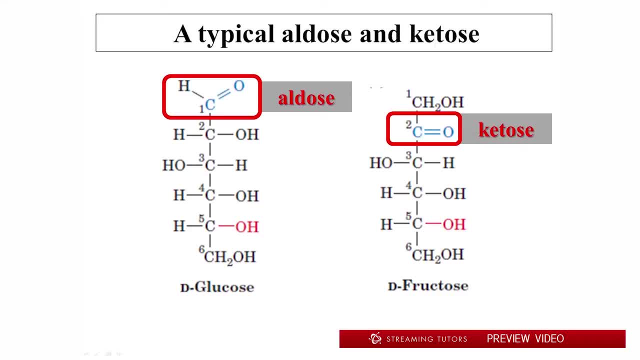 And aldoses have an aldehyde carbonyl group. Ketoses have a ketone carbohydrate group. I'm sorry, carbonyl group. Notice that I've boxed the respective groups here. Glucose is an aldose. It has an aldehyde group. 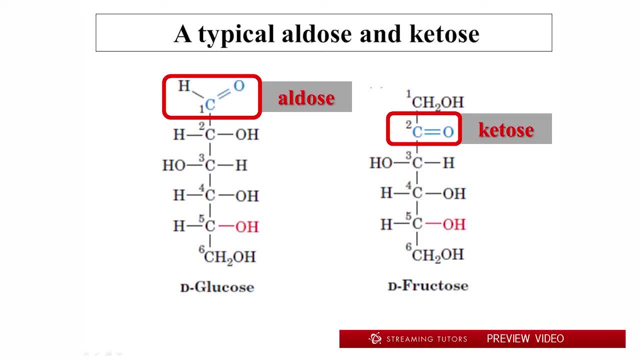 Glucose is a ketose and it has a ketone group, So sugars are often named as ketoses or aldoses. as you'll see over the next few minutes. Let's also look, then, at the numbering scheme. So the numbering scheme is to number the carbon at the end of the linear projection of the structure of the monosaccharide. 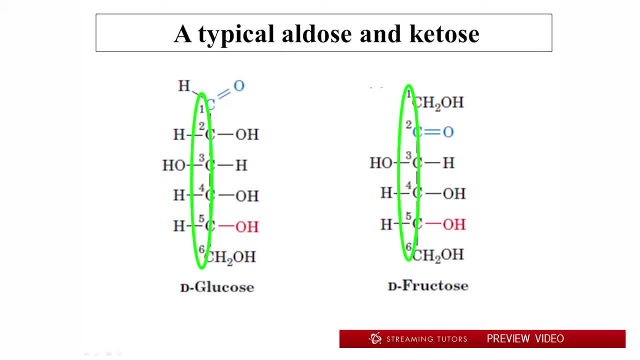 the carbon either containing or nearest to the carbonyl group as the one carbon and then number down from there. So notice the 1.0., The 1.0 through 6.0 numbering of glucose and the 1.0 through 6.0 numbering of fructose. 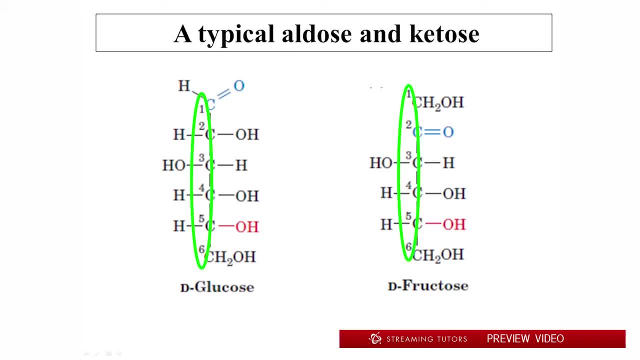 So the one carbon is either the carbonyl-bearing carbon or the one, the terminal carbon, closest to it, as in the fructose case, for example. Okay, Another element of nomenclature. you'll notice the letter D here. 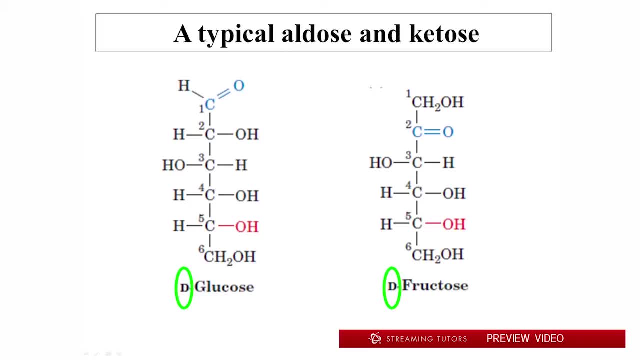 As we talked about extensively in the context of amino acids. biological molecules, virtually without exception, are stereoisomer-specific. They're stereospecific, They're not racemic mixtures of the two stereoisomers. In the case of amino acids, it turns out, coincidentally, that it is the L configuration that is broadly represented. 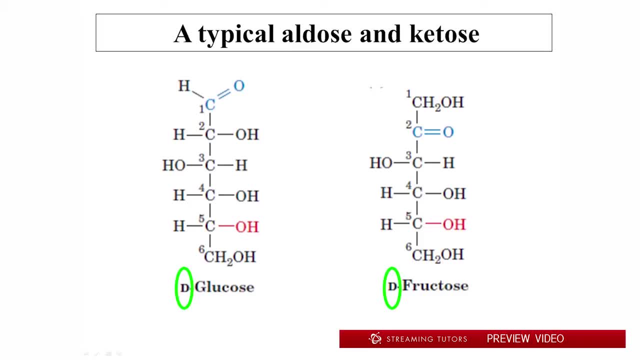 In monosaccharides, the opposite is true. It is the D configuration. L configurations of monosaccharides are quite uncommon, occurring only in specialized circumstances. So when we talk about later in metabolism, we talk about blood sugar, we talk about glucose. 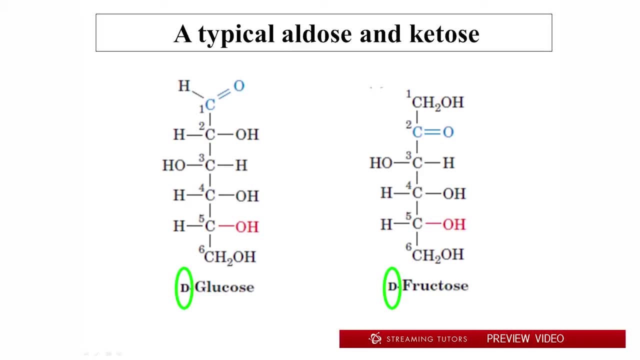 we'll often just implicitly say glucose, knowing that everyone recognizes that we're talking about D glucose unless otherwise specified. Let's talk about where that is Where that nomenclature comes from. So D sugars have, as both D fructose and D glucose here illustrate, have the hydroxyl group on the asymmetric carbon. 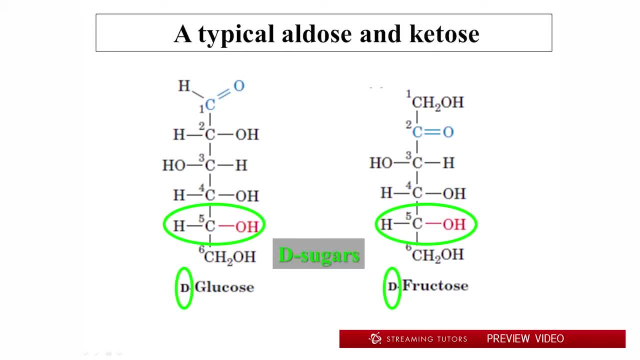 that is, the stereosymmetric carbon, stereospecific carbon rather furthest from the carbonyl group. So in this case it's the 5-carbon in both glucose and fructose. In the Fischer projection the hydroxyl is to the right. 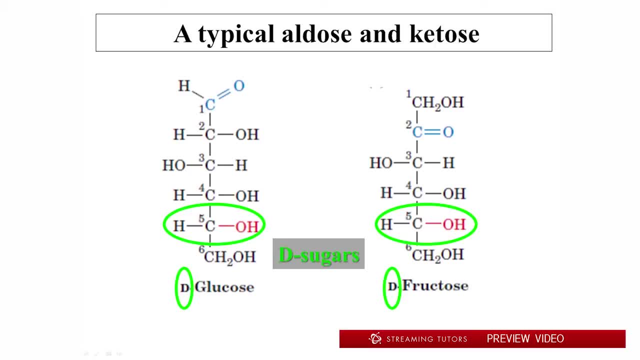 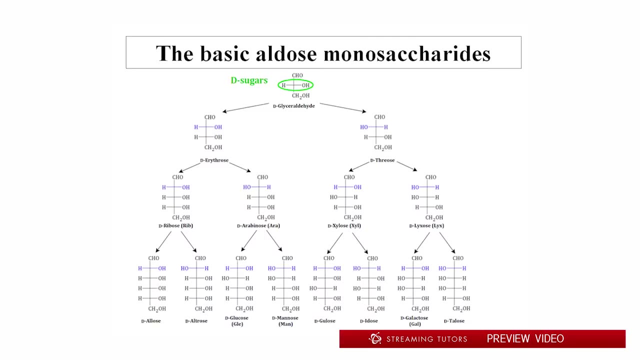 So L Sugars would have this 5-carbon linked hydroxyl group projecting to the left in the Fischer projection. That's its stereochemistry. So let's put this in the larger context of all aldoses first. This really complicated diagram is a little intimidating at first. 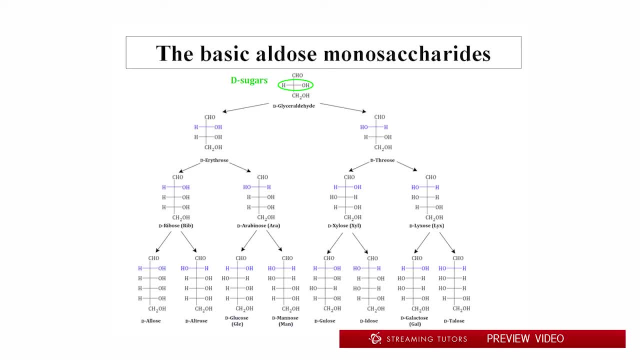 It's actually not as bad as it seems. Let's take a minute and zero in on it and talk through several of the things that we need to pay attention to. So first notice that D sugars, Just like L amino acids, are named relative to the glyceraldehyde stereoisomers that were the original Fischer's original go-to reference compound. 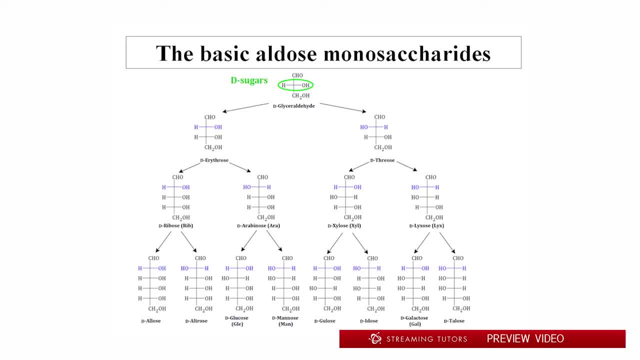 So these compounds are named not for any particular physiological or biosynthetic reason, but just for the organic chemists convenience to be able to organize them mentally with respect to structure. So notice that in the D stereoisomer the Fischer projection thereof of glyceraldehyde. 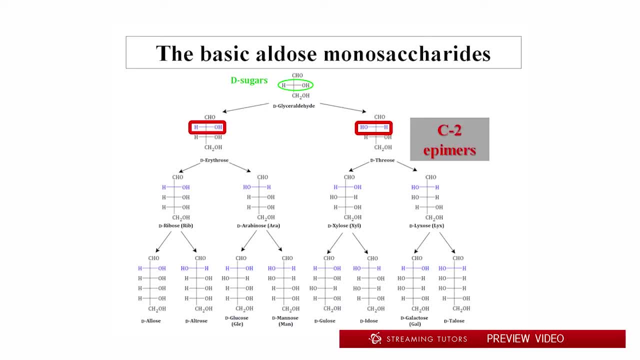 the hydroxyl group projects to the right, as we've talked about, And that's true of all of these D monosaccharides, as you can see, all circled in green here. Let's now look at this organization. 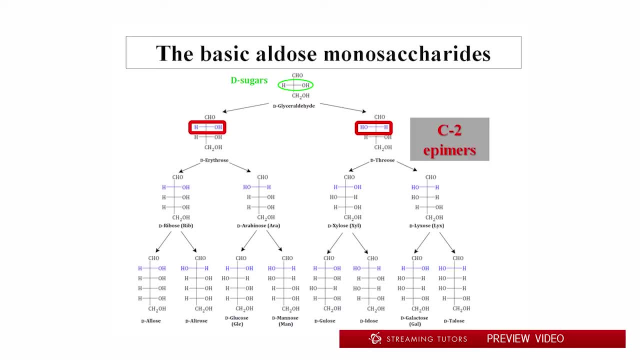 Again, this organization does not imply anything about synthesis or biological function. It's just a human invention to keep track of all of these potential structures. I say potential because most of these structures actually don't occur very often in biological systems and we won't be paying a lot of attention to them. 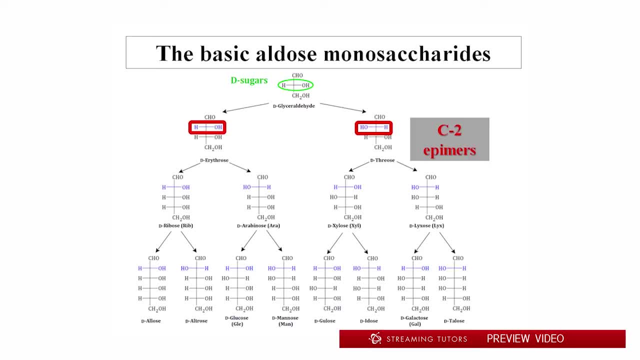 I'll come back and point out to you the few that are important in a moment. But this gives us a chance to introduce a new term: epimers and the change of epimers, called epimerization or epimerization. Notice that the two erythros and threos here differ around the two carbon. 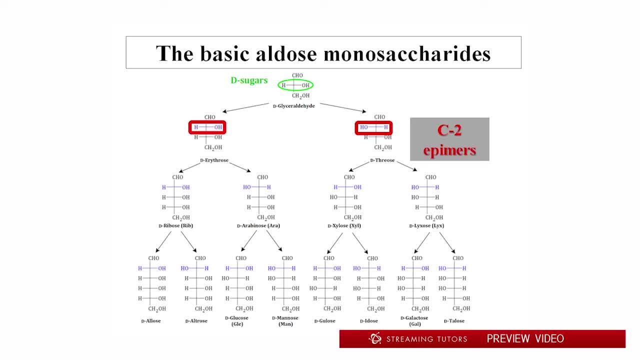 They are two C2 epimers. So they are otherwise identical, except the stereochemistry around C2 is different And D erythros has the hydroxyl group projecting to the right and the fissure projection threos to the left. 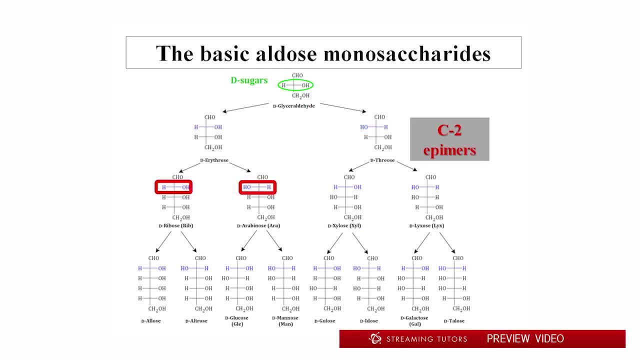 And again the same is true now as we go down to the aldopentoses. We were looking at the aldotreose, the aldotetrose, and now we're at the aldopentose, meaning five carbon aldoses. 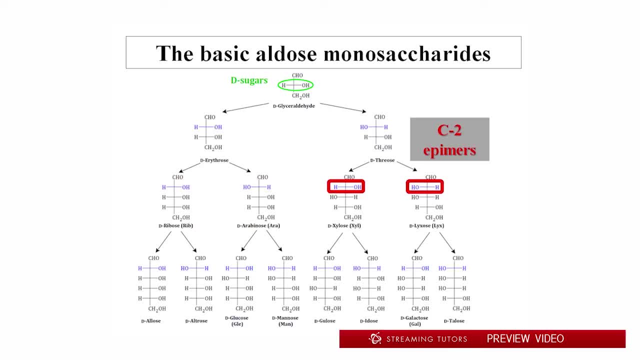 And again notice that each pair is a C2 epimer. Notice that here boxed in red. And then the two pairs are joined by their shared common stereoisomerization around what is now their C3.. What was the C2 of the aldotetroses above? 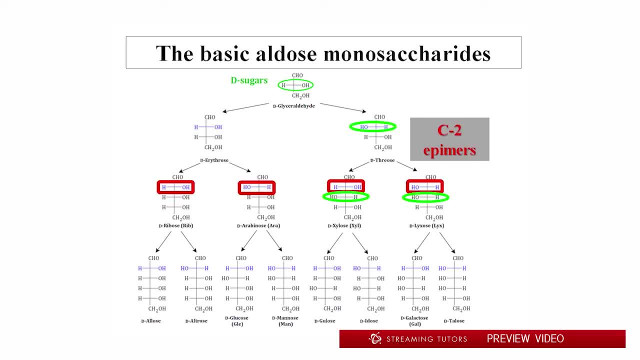 Okay and ditto, over here the same nomenclature. So in other words, these are laid out in an intellectually simple, systematic way. So most biochemical courses you take will not require you to memorize most of these structures. I'll call your attention in a moment to the few that you will want to memorize. 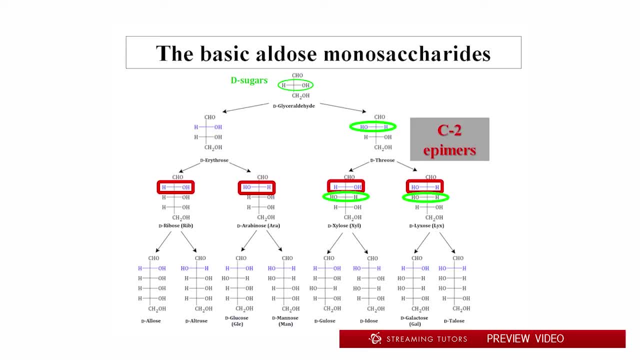 But even if you were in fact tasked with memorizing these structures, if you keep in mind their structural relationships to one another, the memorization of all these aldoses is in fact a quite achievable task, if you in fact needed to do that. 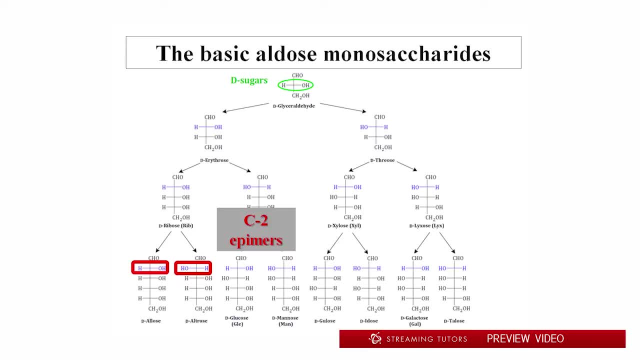 Again we see the same thing now on the next level of order, On the next level of organization, the aldohexoses. These are in fact again C2 epimers Organized in this way, So here organized around a common stereochemistry. 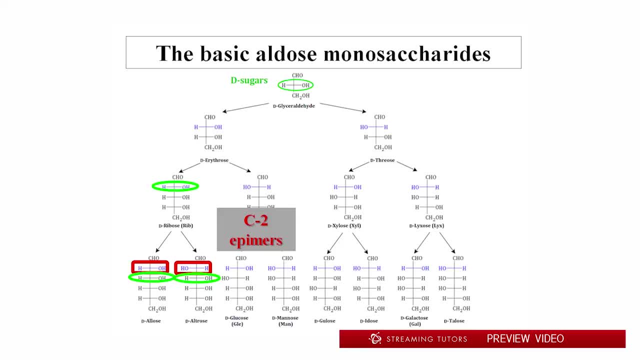 Now around their C3. What was the C2 of the aldopentose sugars above? And the same is true all across the? I won't highlight it here for you, but you might want to print the sheet out and walk through and see that the other pairs of epimers across the aldohexoses behave in exactly the same way. 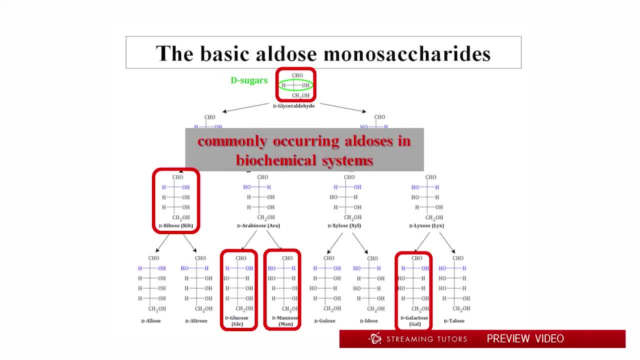 The same way as this pair. Let's now deal with the issue of which ones of these actually play large biological roles, And there are in fact only five of them, and they are boxed here. So glyceraldehyde, typically in a phosphorylated form at the top, plays a role in metabolism. 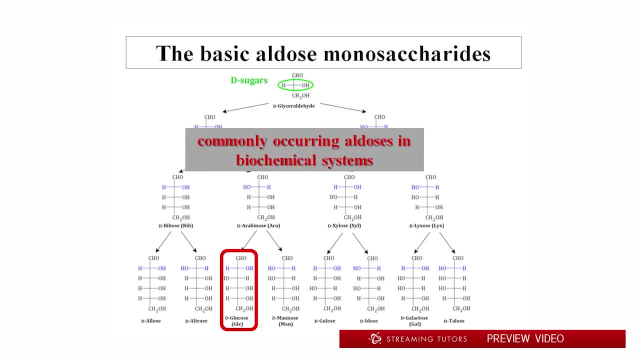 As does glucose at the bottom. In fact, when you talk about blood sugar in metabolism, as we will in the following segments, it is this sugar, D-glucose, that you're talking about. Ribose is important. We'll come to this in more detail in a couple of minutes.